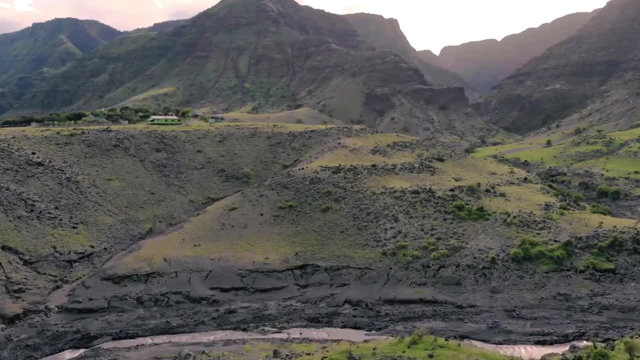 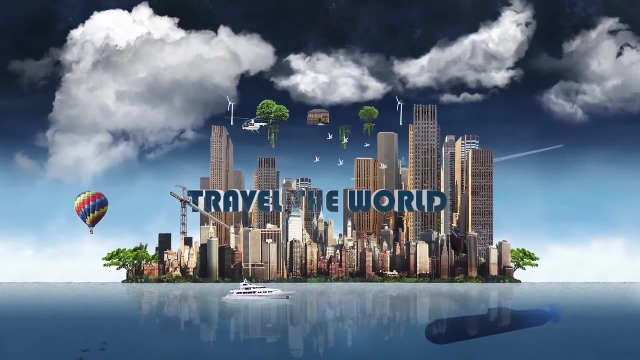 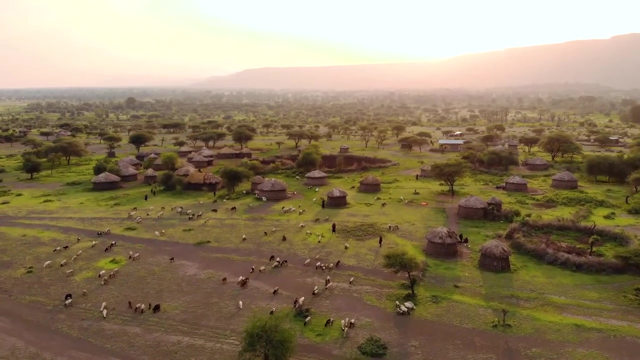 group is Islam, followed by Christianity. Let's check out the 54 countries of Africa, all countries in Africa: 9. How Big Is Africa? Africa is the second largest continent in the world in terms of land area and population. Africa covers a land mass of over 3 million. 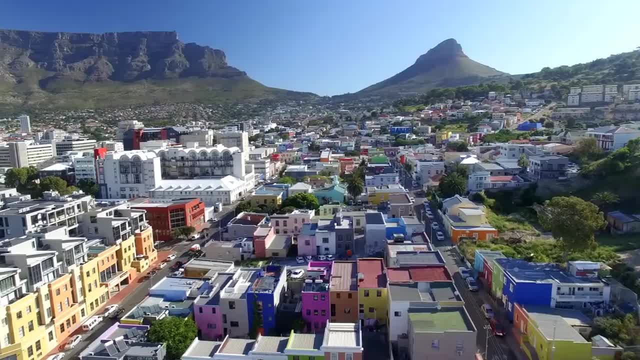 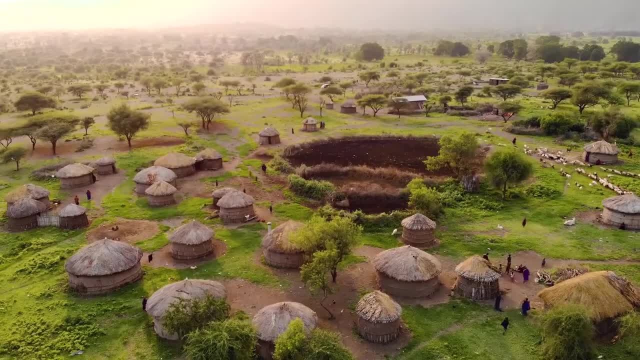 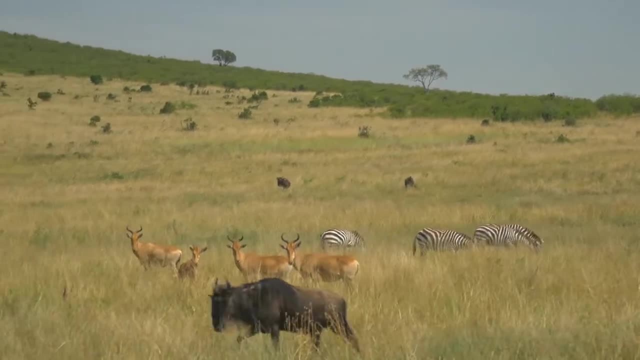 square kilometers, which includes independent island states. Africa is separated from Europe by the Mediterranean Sea and joined with Asia by the Isthmus of Suez, 120-kilometer, 75-mile strip of land which lies between the Mediterranean Sea and the Red Sea. 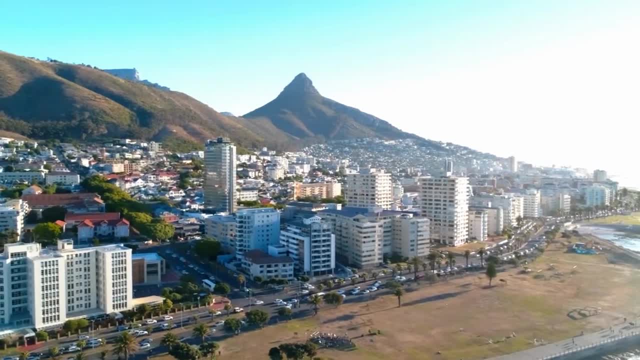 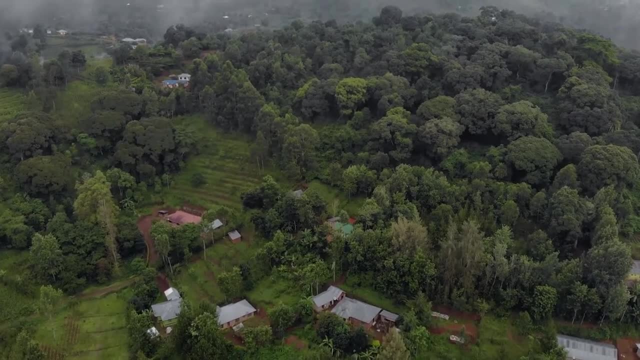 The Suez Rift runs between the Isthmus of Suez, which divides mainland Egypt and Africa. from the Sinai Peninsula, Africa is surrounded by the Red Sea and the Suez Canal in the northeast, the warm Indian Ocean to the southeast, the Mediterranean Sea to the north and the icy-cold. 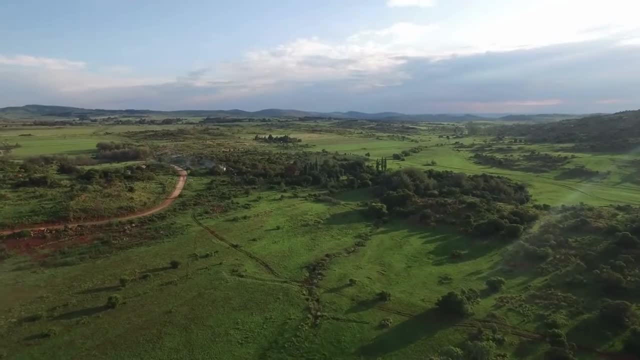 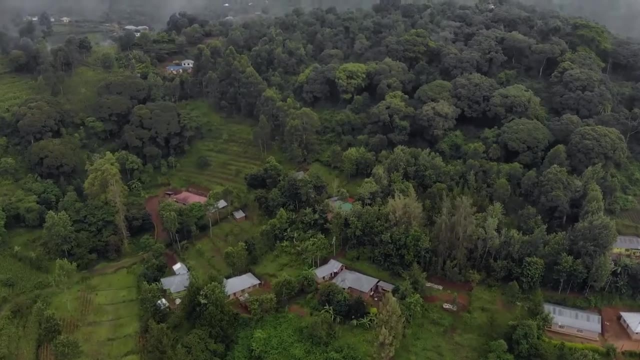 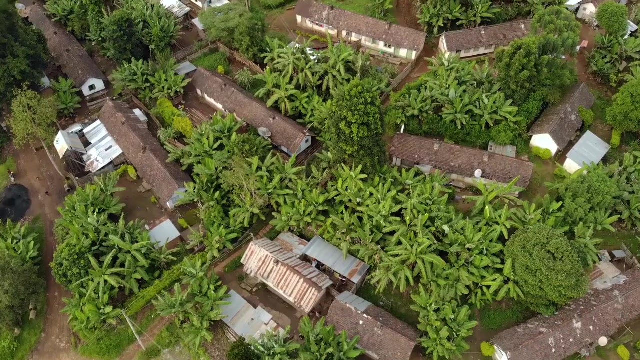 Atlantic Ocean to the west. The distance from the southernmost tip of Africa, at Cape Agulhas, to the northernmost tip at Ras Ben Saka in Tunisia is approximately 8,050 kilometers 5,000 miles. The distance between the most easterly point, at Ras Fun in Somalia, and the 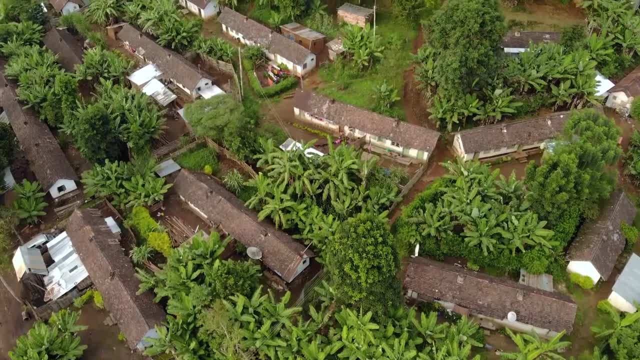 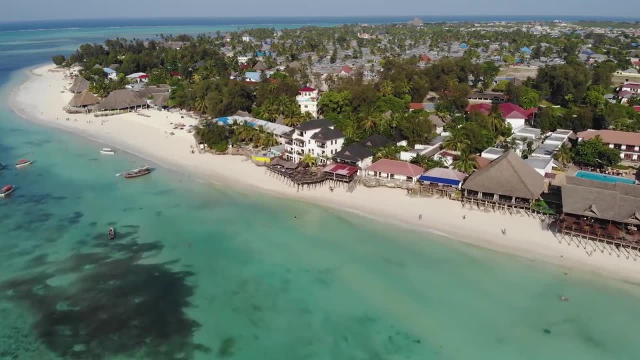 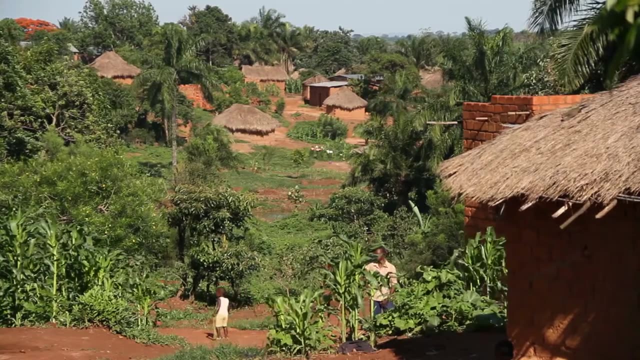 most westerly point in Cape Verde is approximately 7,400 kilometers, 4,600 miles. Africa straddles the equator, which passes through six countries: Gabon, Republic of the Congo, Democratic Republic of the Congo, Uganda, Kenya and Somalia, Surrounded by water from all. 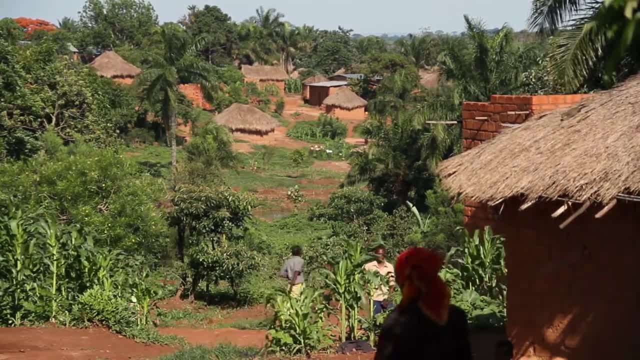 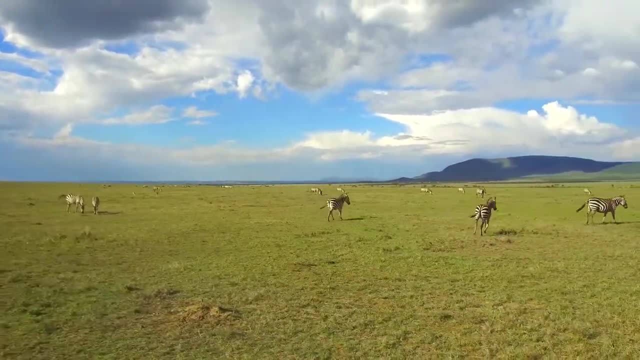 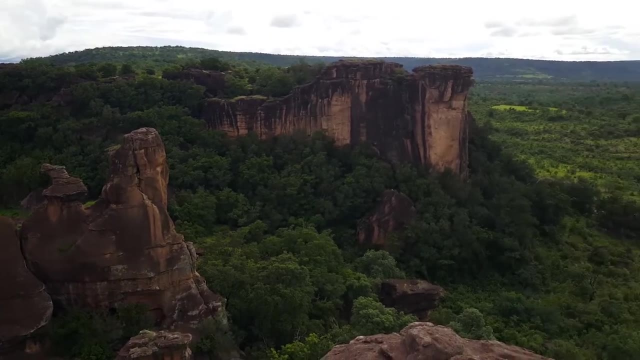 in the northeast is separated from Asia by the Suez Canal and, farther, by the Red Sea. From the east and southeast it is surrounded by the Indian Ocean, from the west by the Atlantic Ocean. The total number of independent states in Africa is 54. The transcontinental country in this 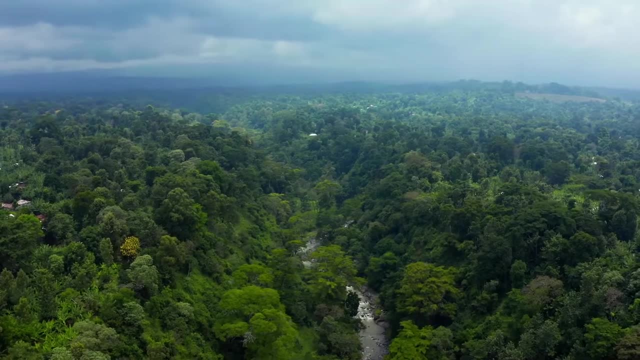 region is Egypt, also having a small part of its territory in Asia, on the other side of the Suez Canal. Africa is surrounded by the Indian Ocean, from the west by the Atlantic Ocean and from the northern Mediterranean Sea in the southwest by the Mediterranean Sea in the eastern Mediterranean. Sea. Among the African countries, the biggest one is Algeria, occupying around 7% of the continent's territory, and the smallest nation is Seychelles, the world-wide famous luxurious beach holiday destination, occupying 115 islands stretching along the mainland's eastern coast. 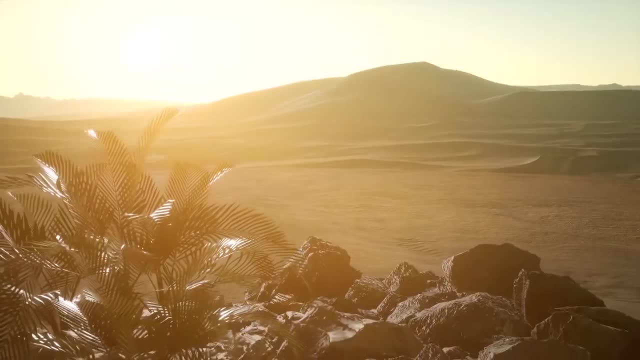 8. Large Countries in Africa by Land Area. The top five largest countries in Africa by land area are: Algeria- covers 6% of the Earth's total surface area and Algeria's largest country by land area. Algeria's largest country by land area. 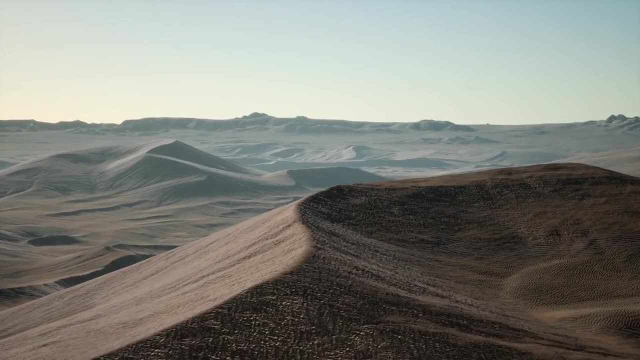 and Algeria's largest country by land area. Algeria's largest country by land area. Algeria's largest country by land area. largest country in Africa and the 10th largest in the world. The Democratic Republic of the Congo, landlocked country in Central Africa. 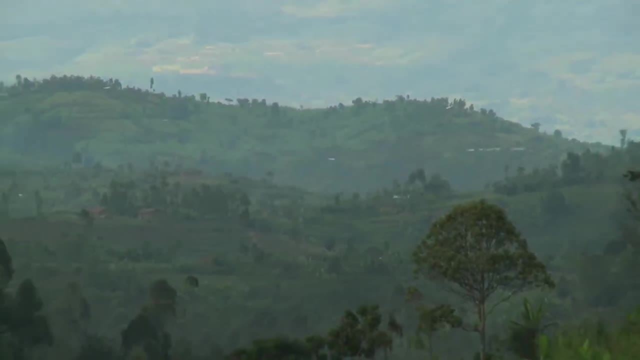 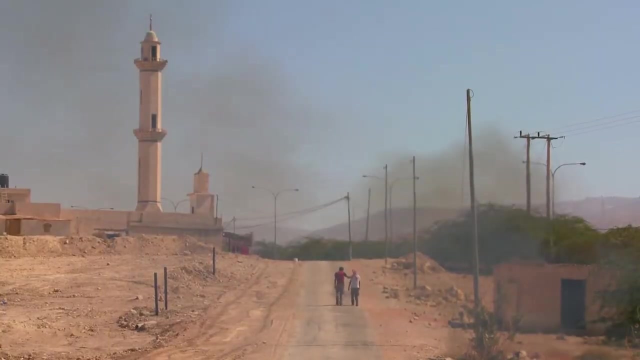 larger than the combined land area of Norway, Sweden, Germany, France and Spain. Sudan in North Africa, sharing a coastal border with the Red Sea. Libya in North Africa, sharing a coastal border with the Mediterranean Sea. Chad landlocked country in North Central Africa. 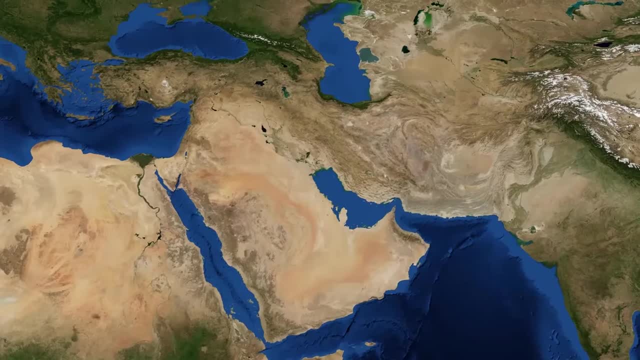 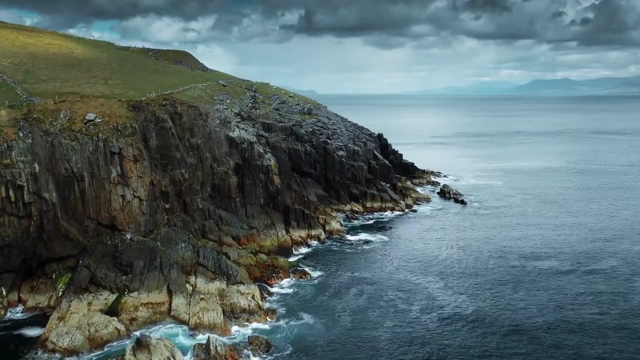 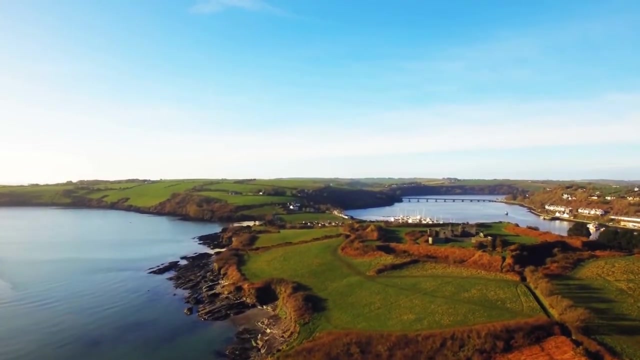 largest and smallest countries in Africa by land area. The top five smallest countries in Africa by land area are all island nations: Seychelles, an archipelago of 115 islands in the Indian Ocean. Sao Tome and Principe, two main islands of the archipelago, located in the Gulf of Guinea. 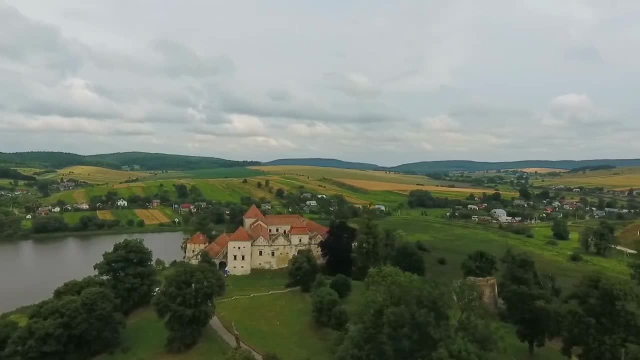 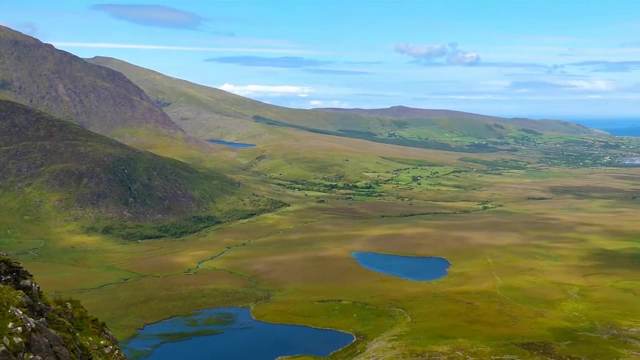 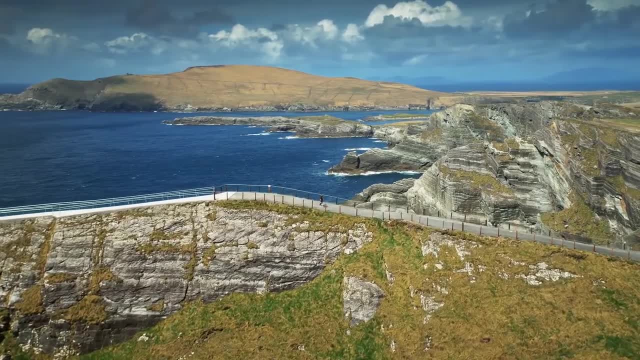 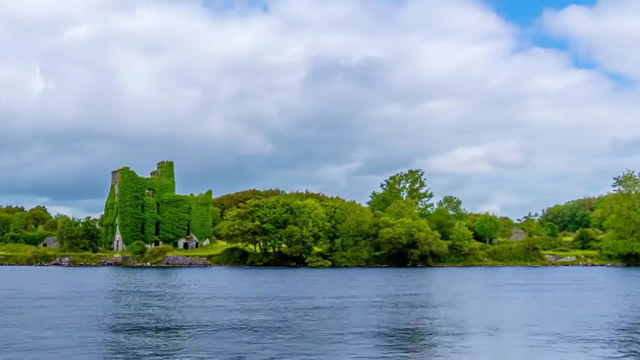 Cape Verde archipelago of the Indian Ocean. Cape Verde, archipelago of 10 islands located in the Indian Ocean. The smallest country in mainland Africa is the Republic of Gambia. It is almost completely surrounded by Senegal, except for its western coastline along the Atlantic. 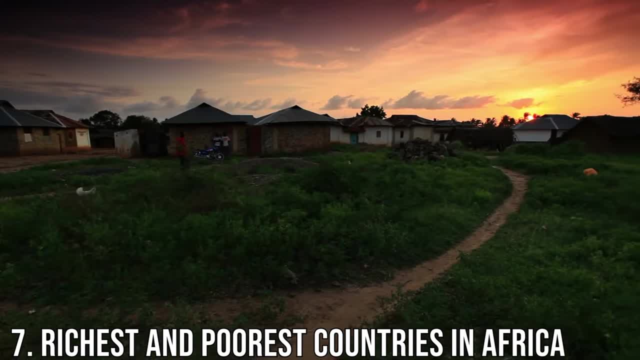 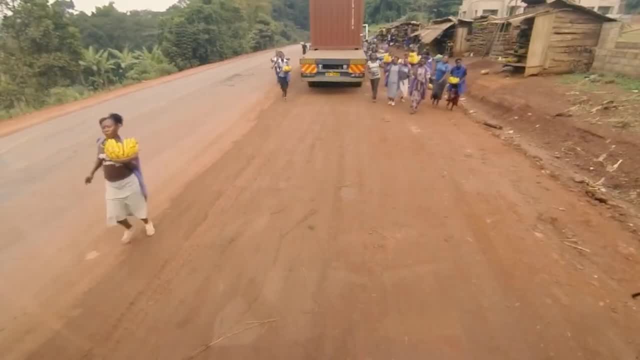 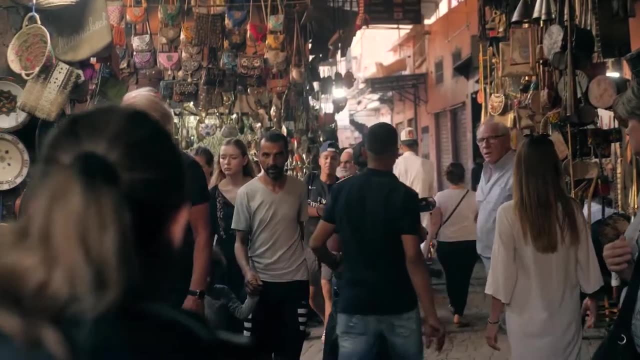 Ocean. 7. Richest and poorest countries in Africa. Looking at the purchasing gross domestic product of the countries in Africa, the top five richest countries in Africa in 2019 were Egypt, Nigeria, South Africa, Algeria, Morocco. The top five poorest countries in Africa in 2019 by purchasing GDP were Burundi. 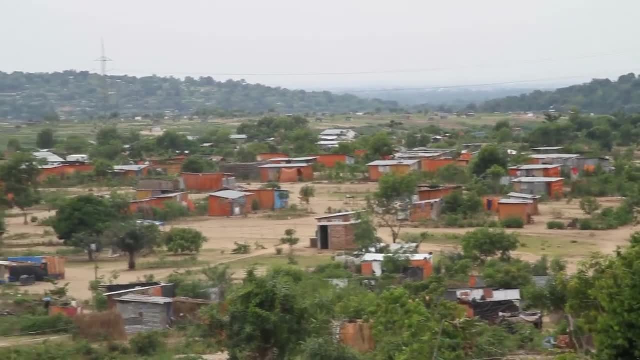 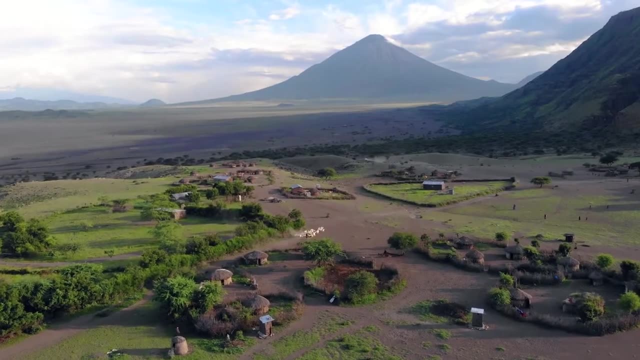 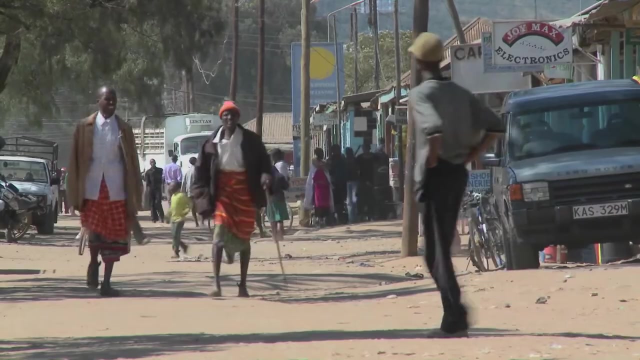 the Central African Republic, the Democratic Republic of the Congo, Eritrea, Liberia. 6. Northern Africa: Northern African countries: Algeria, Egypt, Libya, Morocco, Sudan, Tunisia. Northern Africa has a population of more than 249 million and contains six different countries. 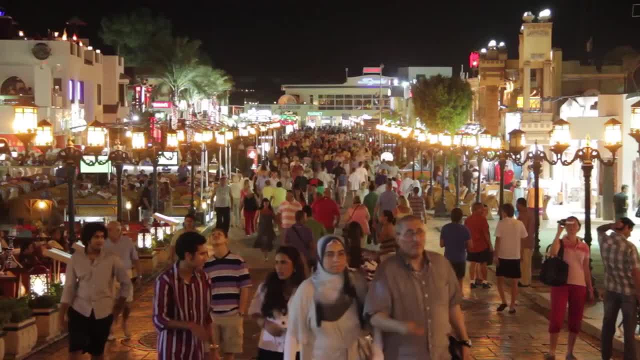 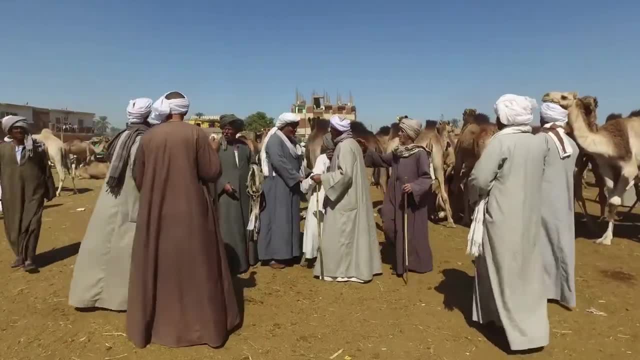 The most populous country in Northern Africa is Egypt, which has a total population of more than 102 million. The least populous country in the subregion is Libya, with around 6.87 million people. All the countries of Northern Africa identify themselves as Arab and Muslim countries. 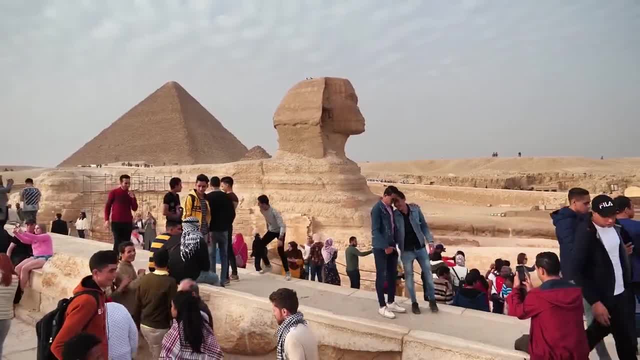 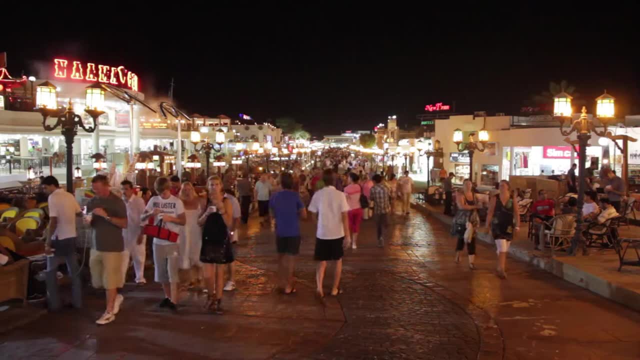 Hence, most of the people in these countries speak Arabic and practice the religion of Islam. Cairo, the Egyptian capital, is the most populous country in the subregion, with a population of more than 20 million. Other large cities in the subregion include: 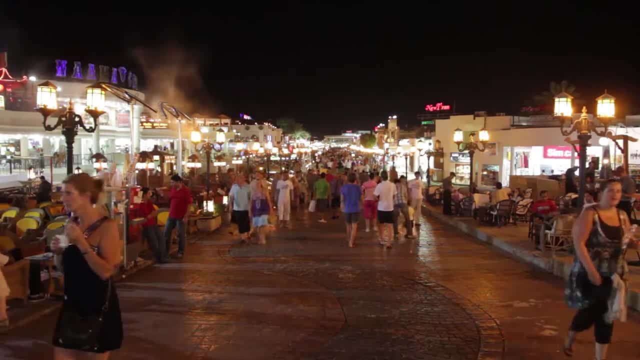 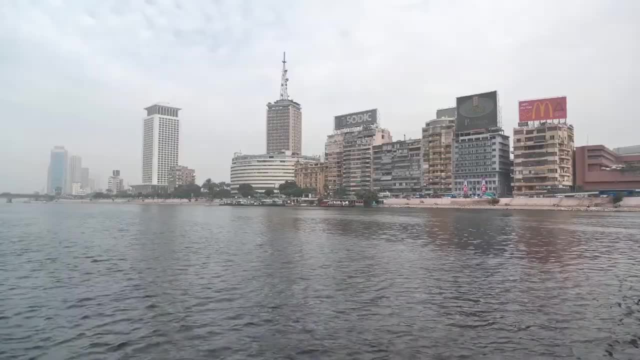 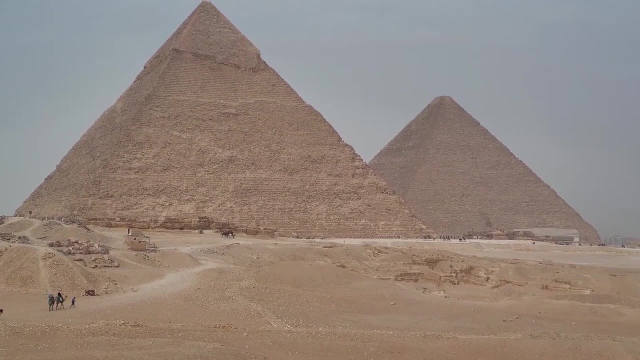 Egypt's Alexandria and Morocco's Casablanca. 5. Eastern Africa: This includes Burundi, Comoros, Djibouti, Eritrea, Ethiopia, Kenya, Madagascar, Mozambique, Malawi, Mauritius, Rwanda, Seychelles, Somalia, South Sudan, Tanzania, Uganda, Zambia and Zimbabwe. Eastern Africa contains more than 453 million people living in 18 different countries. The subregion's most populous country is Ethiopia, with a population of nearly 115 million. The least populous country in Eastern Africa is the island country of the Seychelles. 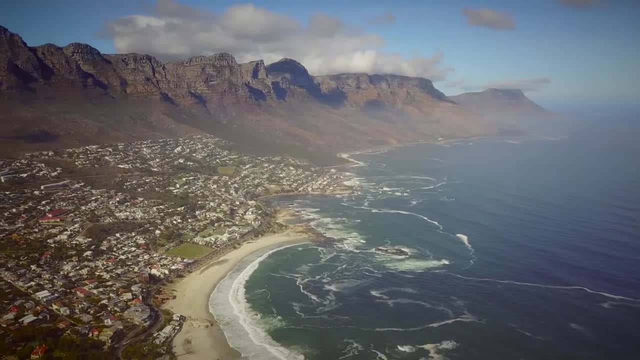 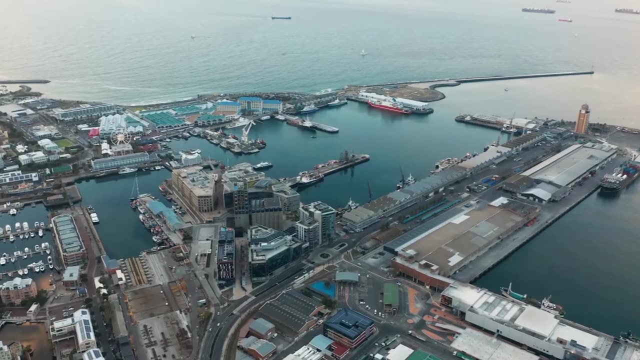 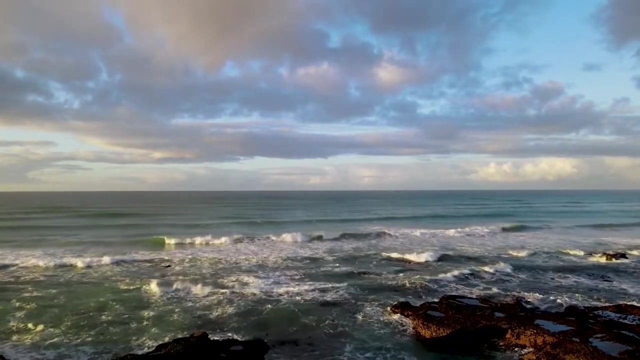 4. Western Africa. This includes Benin, Burkina Faso, Cabo Verde, Gambia, Ghana, Guinea, Guinea-Bissau, Ivory Coast, Liberia, Mali, Mauritania, Niger, Nigeria, Senegal, Sierra Leone and Togo. The region of Western Africa is home to. approximately 409 million people living in 16 different countries. The most populous country in the subregion is Nigeria, which is also the most populous country in Africa and the seventh most populous country in the world. The country has a total of over 206. 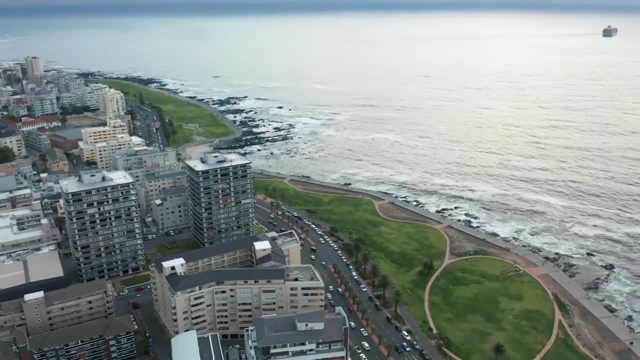 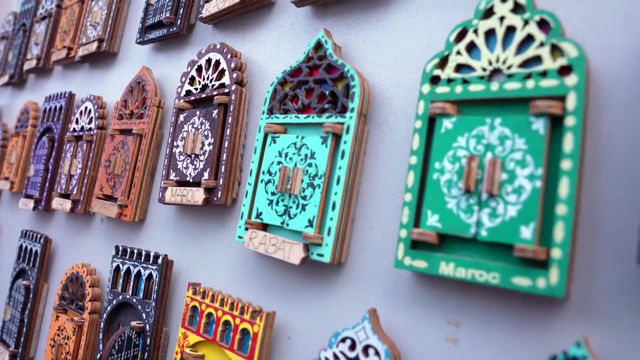 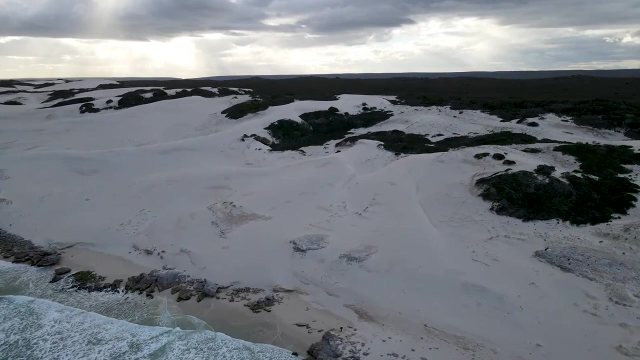 million people. The least populous country in the subregion is Cape Verde, which is an island nation lying off the coast of Western Africa. It has less than 556,000 people. Western Africa contains a vast number of ethnic and linguistic groups. Islam is the most dominant religion of the subregion. 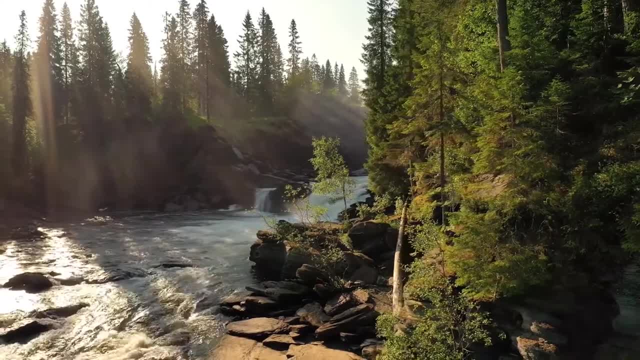 especially in the north. It is the most dominant religion in the region, especially in the north, While Christianity generally dominates the southern part of the region's southernmost countries. Western Africa was once the home of vast empires, including Ghana and Mali. 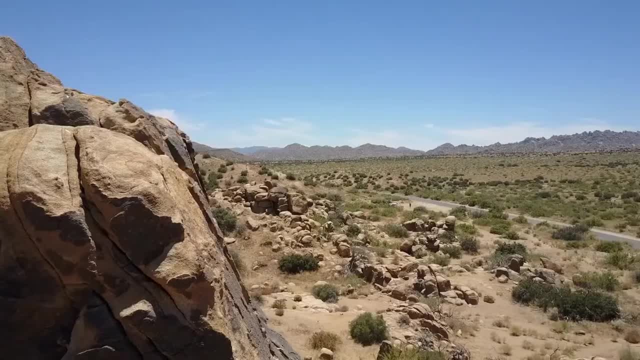 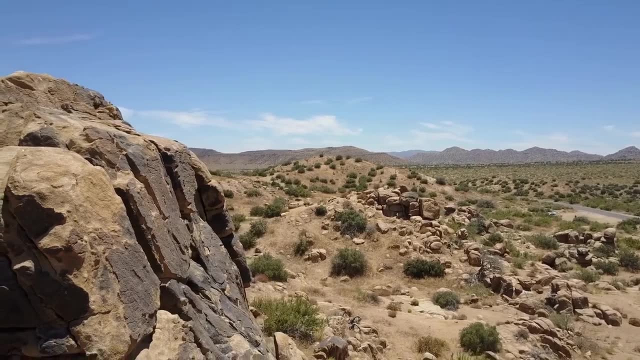 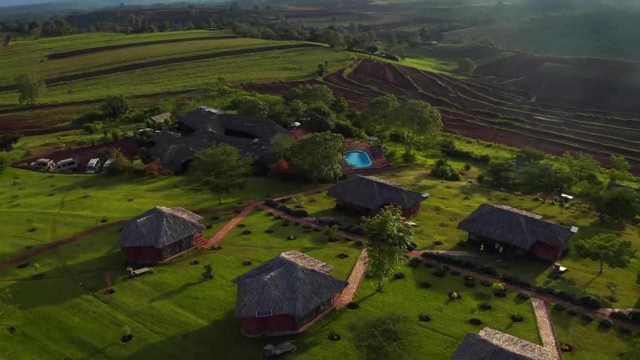 which are now the names of two of the subregion's countries. The most populous city in Western Africa is Lagos, the former capital of Nigeria, which is home to about 21 million people. 3. Middle Africa: This include Angola, Cameroon, Central African Republic, Chad, Congo, DR Congo. Royal Guinea, Gabon, Ceutum and Prinsip. More than 183 million people live in Middle Africa's nine different countries. The subregion's most populous country is the Democratic Republic of the Congo, where more than 89 million people live, The subregion's least populous country. 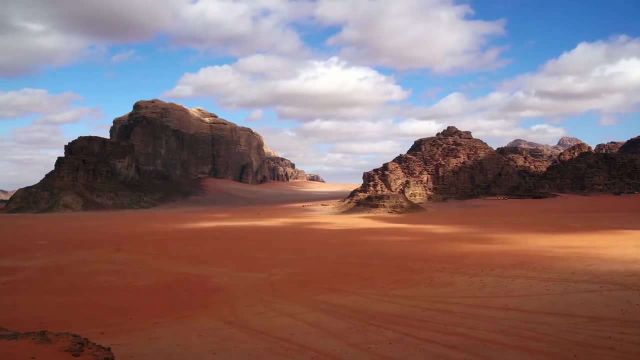 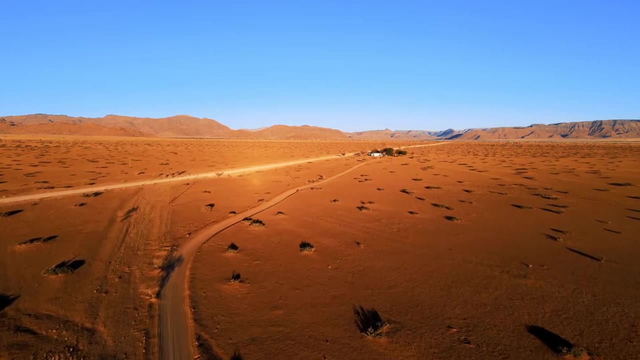 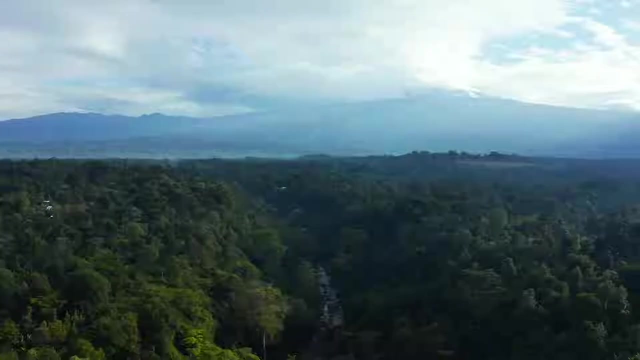 Ceutum and Prinsip, which can be found off Middle Africa's West Coats, contains around just 209,000 people. The subregion's biggest city is the capital of DR Congo, Kinshasa. It boasts a population of 13.3 million, making it the third most populous city in Africa. 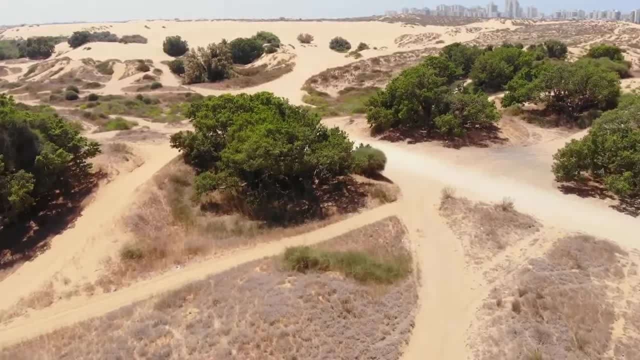 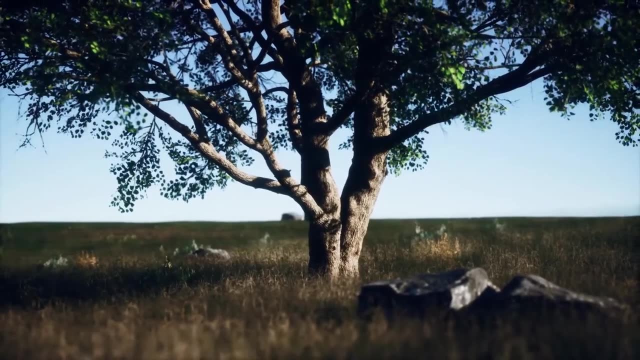 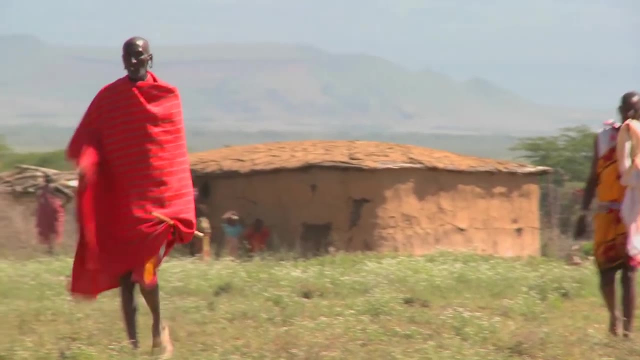 Africa's fourth most populous city, Luanda. the capital of Angola is also located in Middle Africa. 2. Southern Africa: This include Botswana, Eswatini, Lesotho, Namibia, South Africa. South Africa's population is an estimated 68 million people. 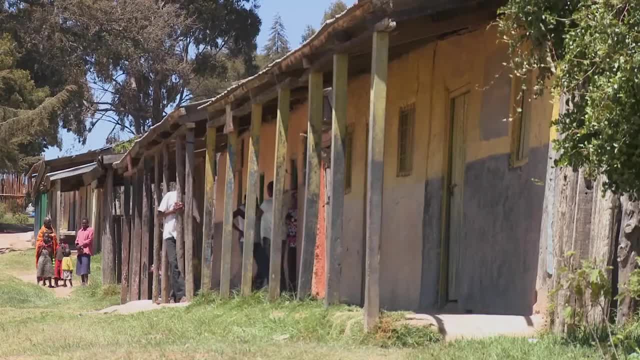 making it the least populous of all of Africa's subregions. Most of these people live in just one subregion. The population of South Africa is about 16,000 people, while the population of the Middle African subregion is about 1,000,000.. In the Middle African subregion, 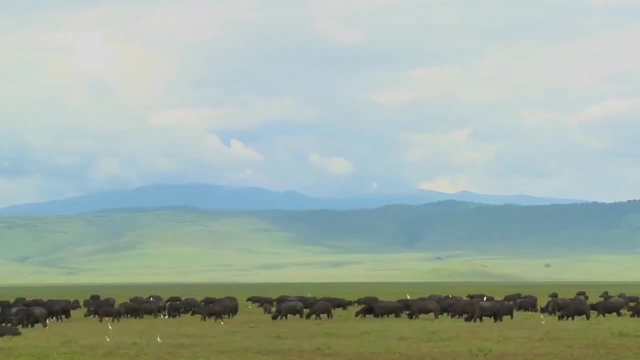 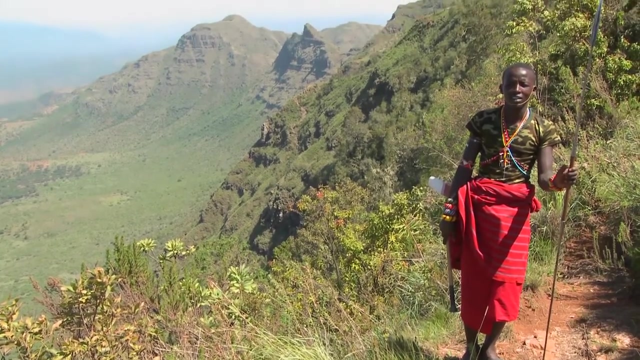 of the subregion's five countries, South Africa, which has a total population of around 59 million people. Southern Africa's least populous country is the landlocked country of Eswatini, also called Swaziland, with a population numbering approximately 1.1 million people. 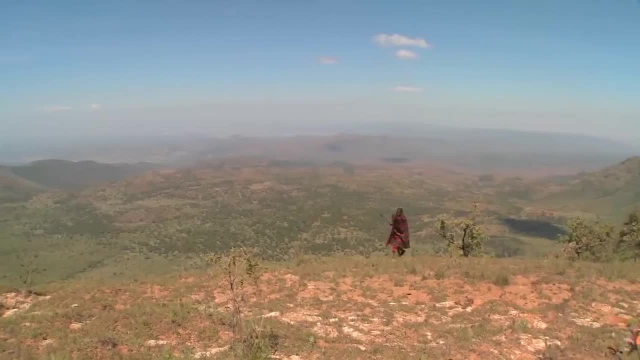 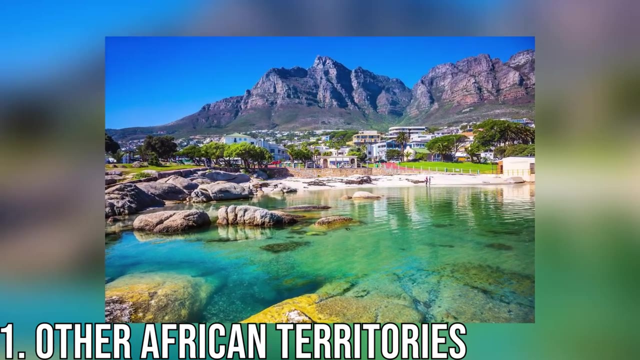 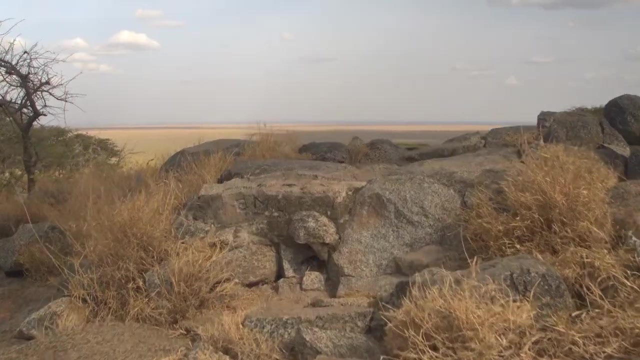 Southern Africa's most populous city is Johannesburg, which is located in South Africa and is home to around 4.4 million people. 1. Other African Territories. In addition to 54 countries, Africa also includes three dependencies and one disputed territory. Two of the dependencies, Réunion and Mayotte, are controlled by France. Réunion is an island. 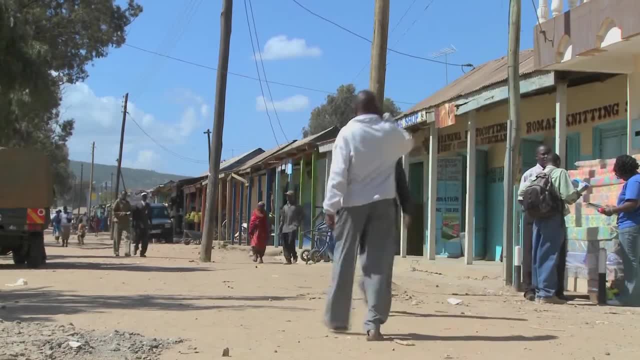 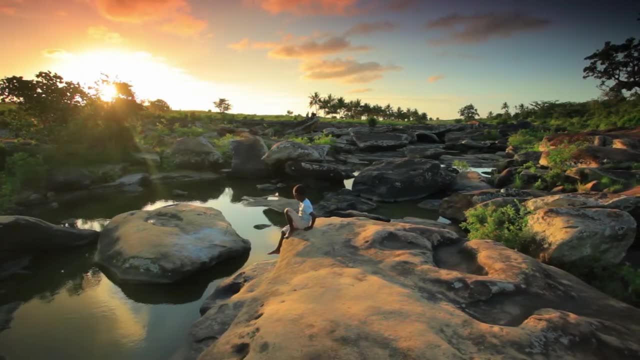 located just west of the small island country of Mauritius and east of the large island country of Madagascar. It is the most populous of Africa's dependencies, containing approximately 895,000 inhabitants. Mayotte is located in the Comoros Islands, off the coast of Mozambique and borders. the country from the north to the south. Réunion is the most populous city in the country, known as the Comoros. The least populous territory in Africa is the British-controlled dependency of St Helena, which is located far off the coast of Middle Africa, practically in. 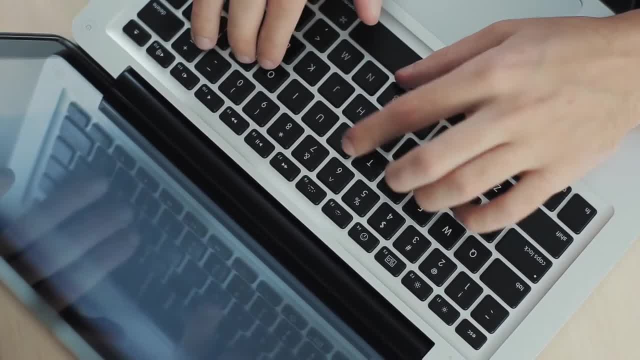 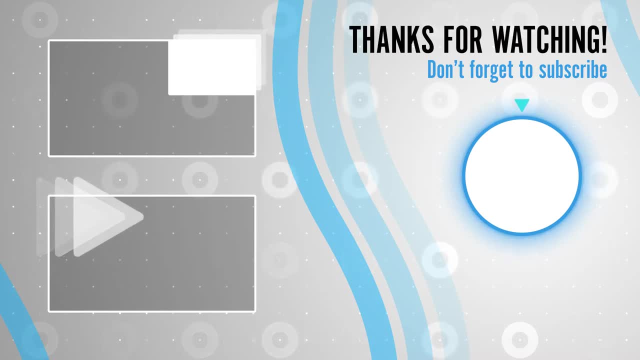 the middle of the South Atlantic Ocean. Do let us know in the comments if you want to visit any of these countries. Please subscribe to Travel the World. Thanks for watching. See you in the next video.